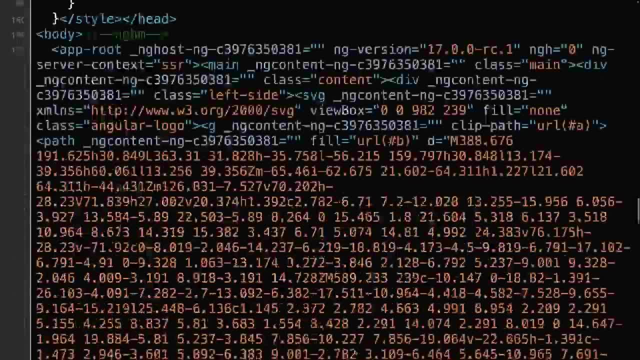 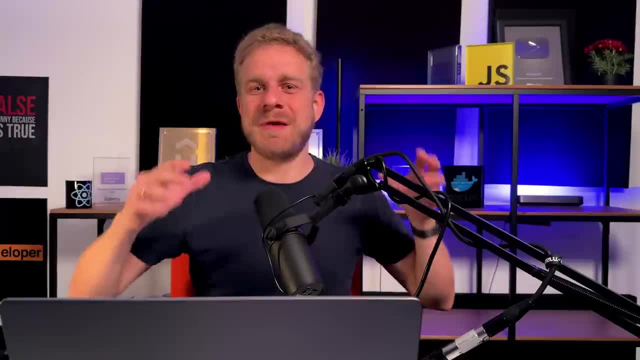 Instead, it just works, as you can see, if you visit the website, because there you'll then get that pre-rendered content instead of an empty HTML page, And that, of course, is great for search engine optimization. And what's even better is that all that server-side rendering stuff. 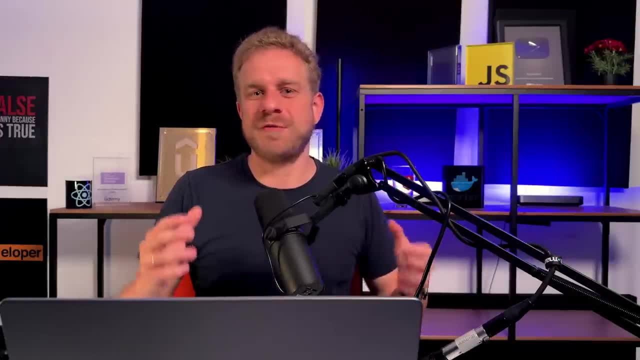 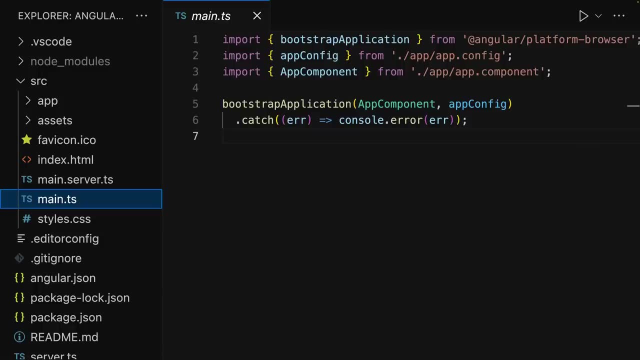 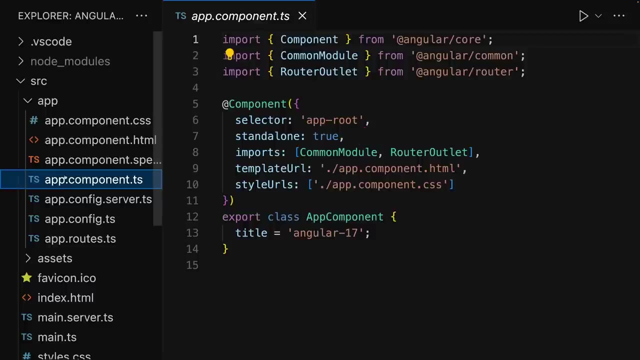 happens in a very efficient and thoughtful way, making sure that your Angular apps are served as quickly and performantly as possible. But that's not all that changes when you create an Angular project. Instead, you'll also notice that now, by default, Angular projects come with standalone components being enabled as a default. 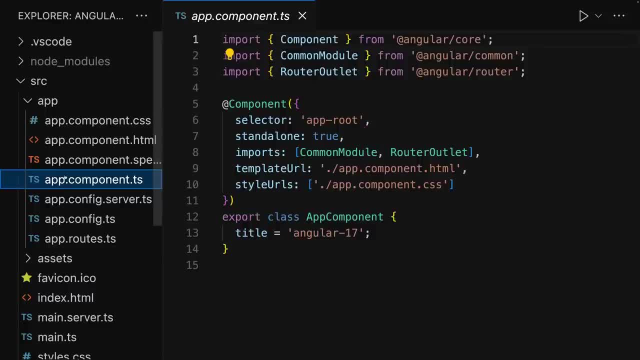 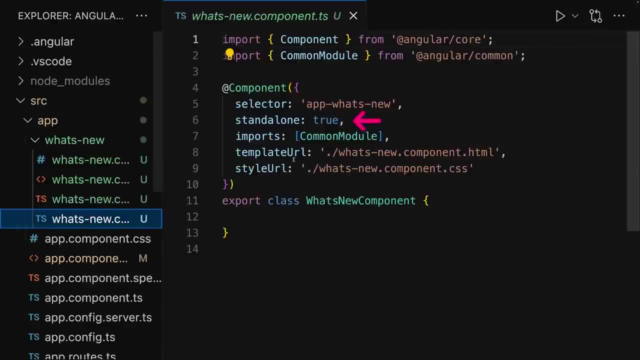 So therefore, you'll see that the app component you got in a new project is a standalone component, And if you generate new components in the project, those will also be standalone components, Though of course, you can also easily change that and override that if you want to stick to modules. 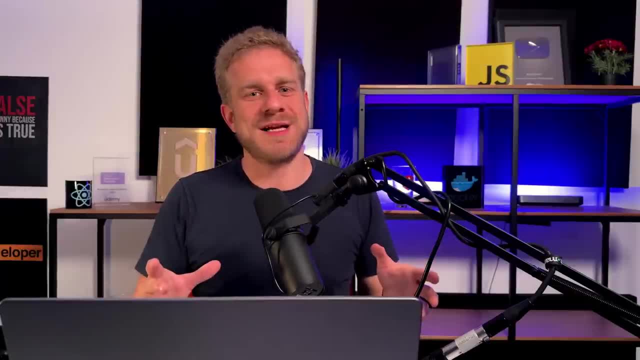 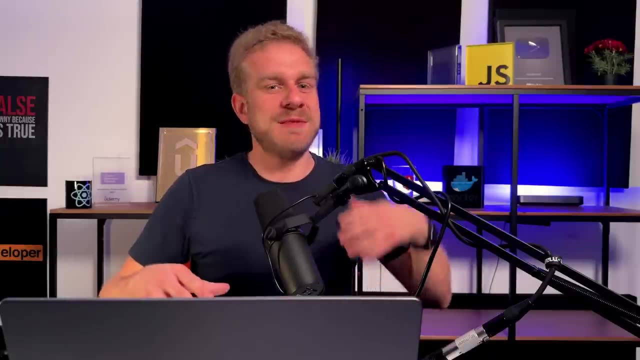 And this is now probably a good time to also mention and emphasize that, whilst Angular gives us all these exciting features and all these new features, it's worth noting that the majority of Angular projects, especially established, big, mature projects, will not use all these features yet. 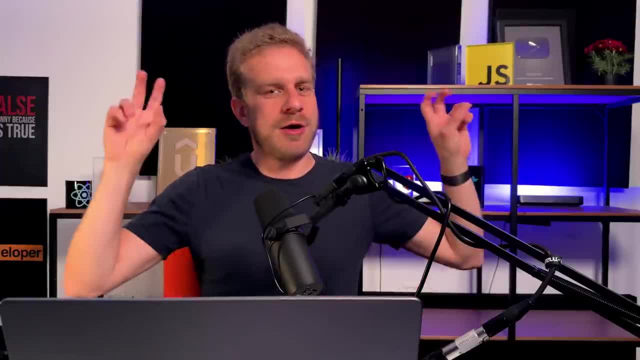 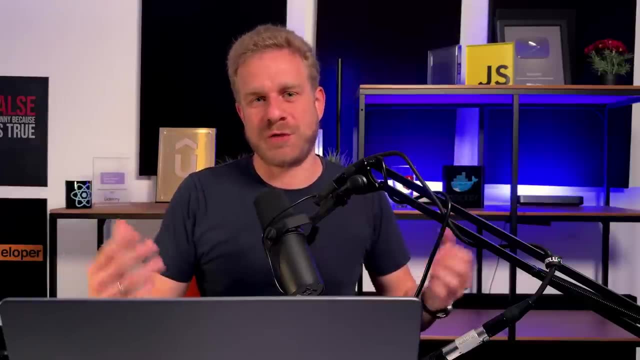 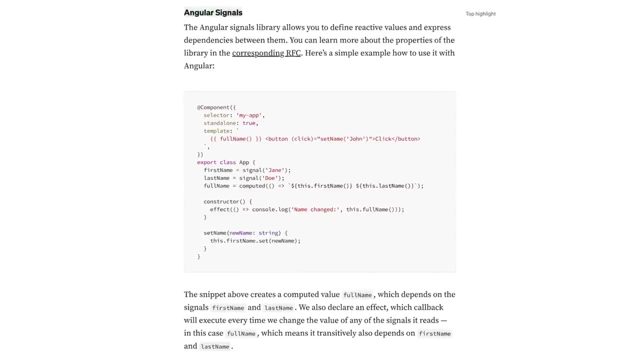 So at the moment, it's definitely also a good idea to learn the old Angular and not just the shiny new stuff, even though the shiny new stuff will, of course, be important in the future of Angular. Now, speaking of that future, it definitely also includes signals, a feature introduced with Angular. 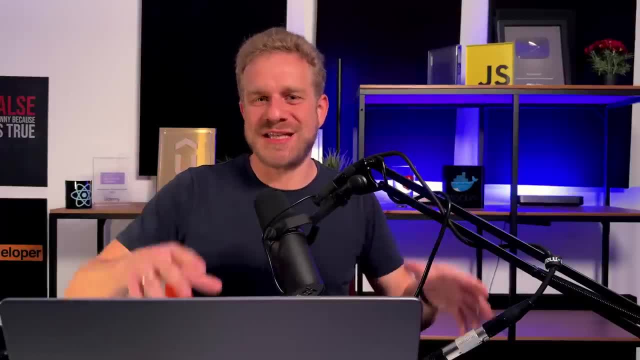 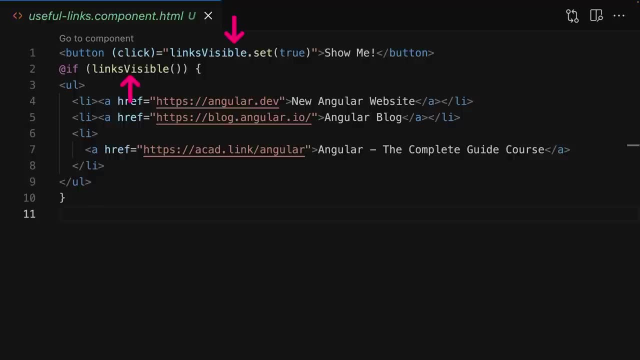 16.. In short, signals give you a different way of managing state, so data that changes over time in your Angular applications And now with Angular 17,. signals are stable, though there also are more signal-related features to come in future Angular versions. 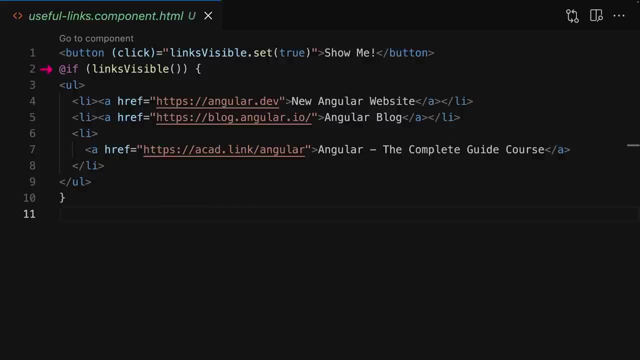 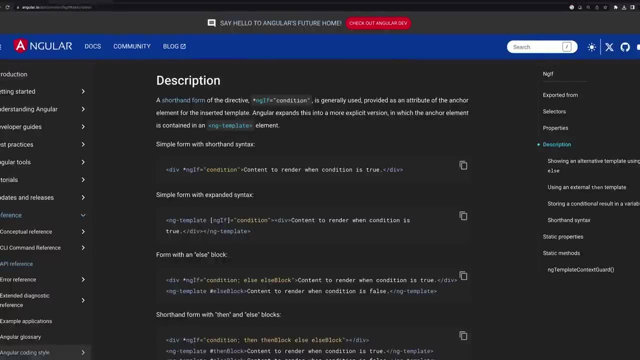 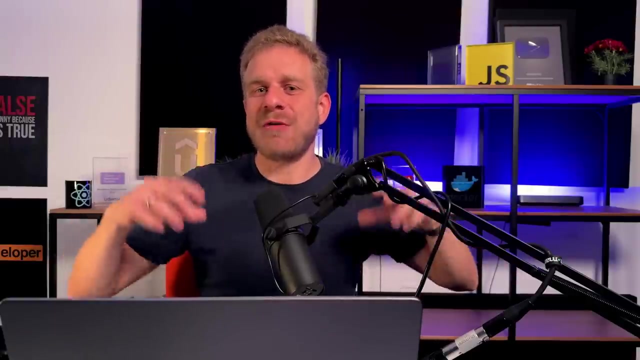 And what's this if thing here we see on the screen? Well, that's also a brand new Angular feature, a brand new template control flow syntax. You no longer have to use the ng-if, ng-for and ng-switch directives- even though you still can, of course- But instead there's now a new built-in. 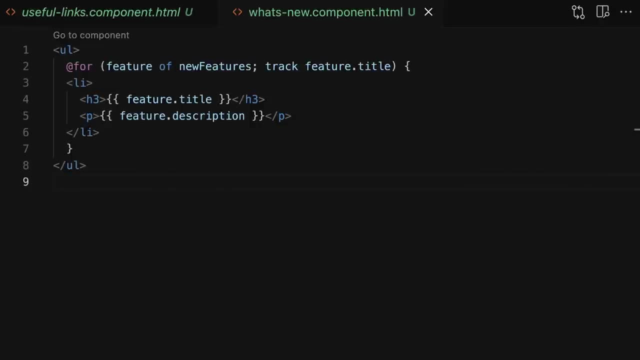 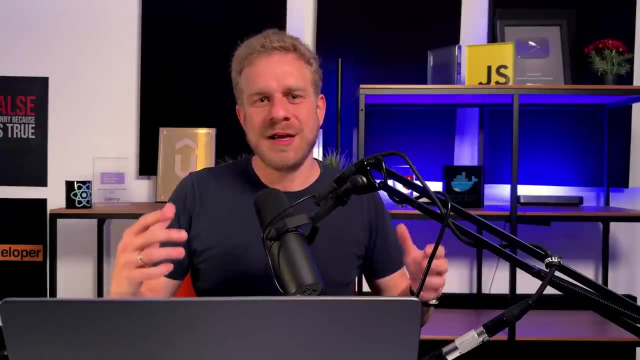 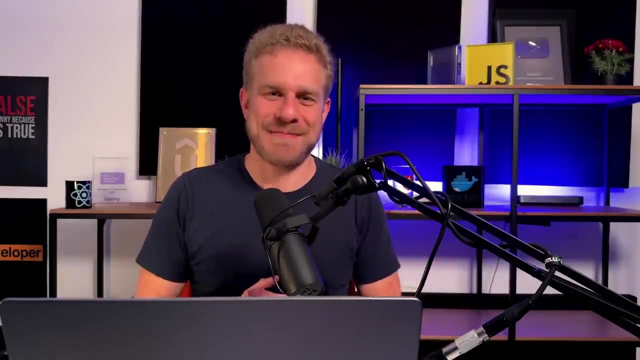 syntax which you can use in your Angular templates without importing anything or without any extra configuration, And this new syntax therefore also gives you an easier, leaner and, as it turns out, also a bit more performant way of handling conditional or list content in your templates.